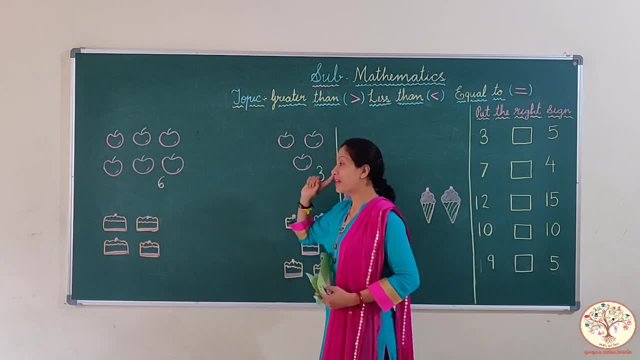 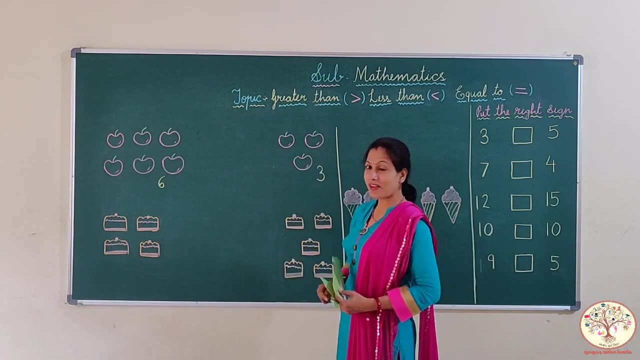 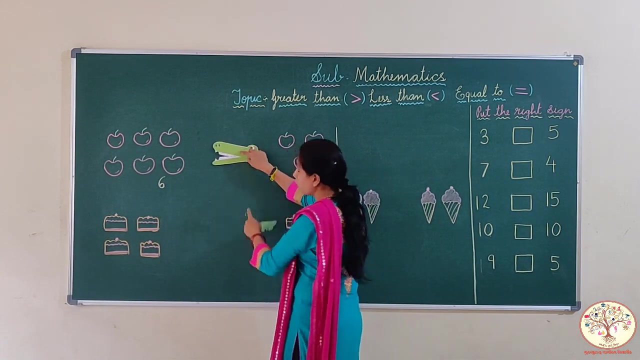 More apples. Six is bigger number than three, So six apples are more than three apples. Cuckoo will eat six apples. And look at the Cuckoo's mouth. Where is Cuckoo's mouth open Towards more apples. 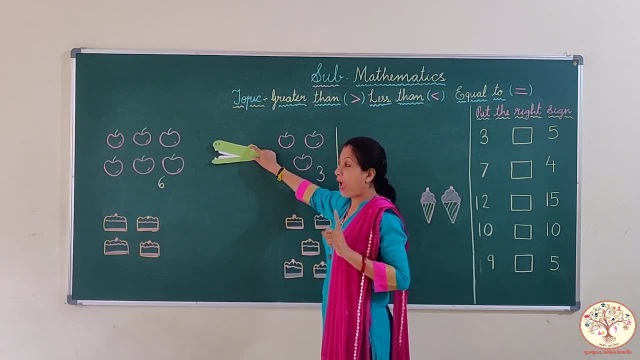 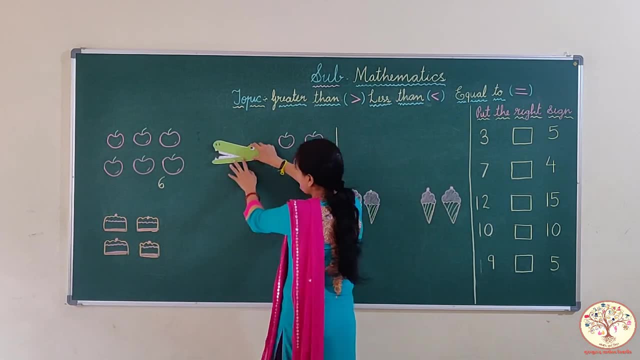 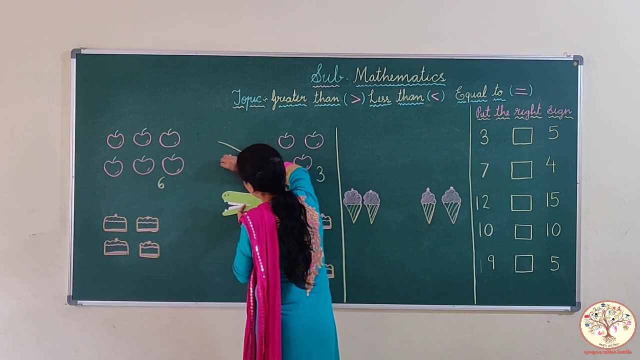 Because Cuckoo's remains always hungry and it eats more thing, bigger number. Ok, So when we put the sign of Cuckoo's mouth in our notebook, we put it like this: This is Cuckoo's mouth, Ok. 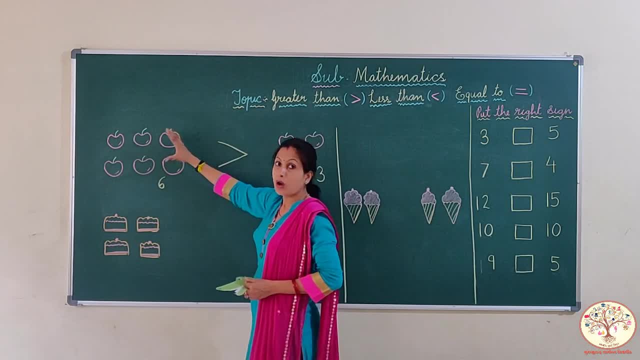 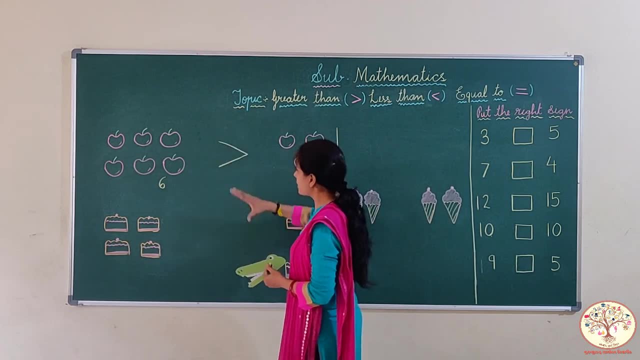 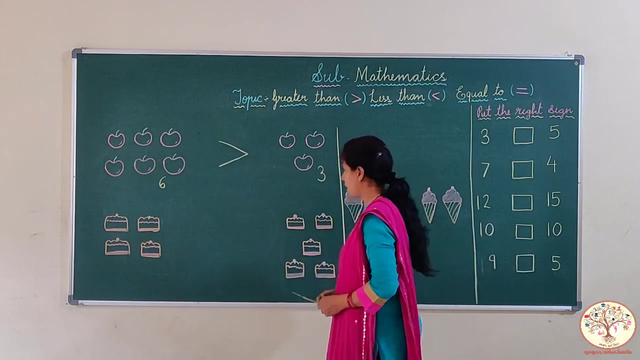 The wide open area remains always towards more things. Ok, So this is the sign towards more things. Do you feel like this is Cuckoo's mouth? This is Cuckoo's mouth. More apples are going to be eaten. Cuckoo has eaten apples. 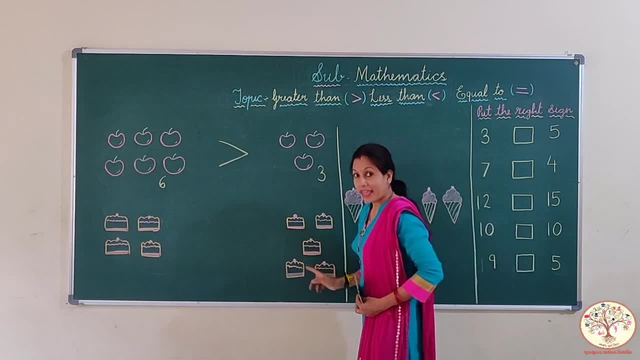 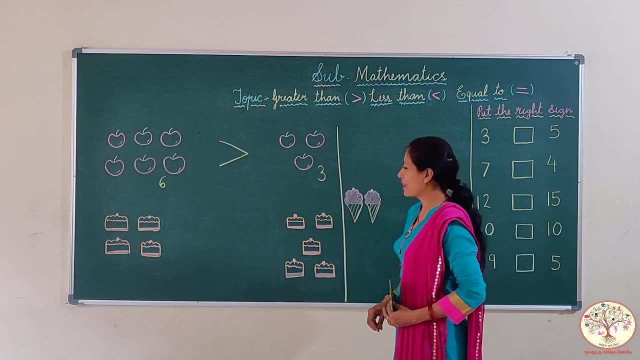 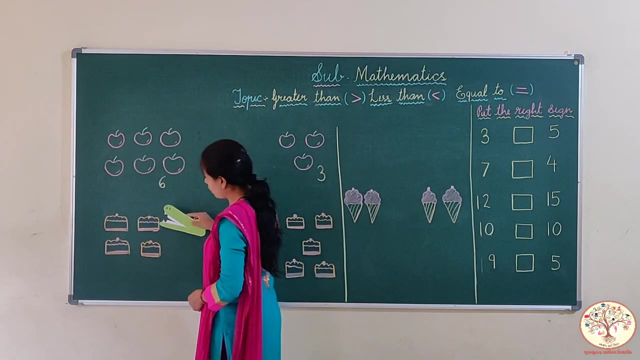 Now he looks cakes. Ok, And let's count which group is more Ok, Which group has more cakes? More cakes, Let's count. Cuckoo is counting You two. count them One, two, three, four. 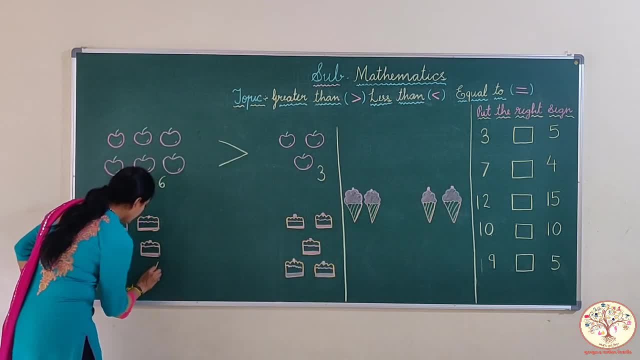 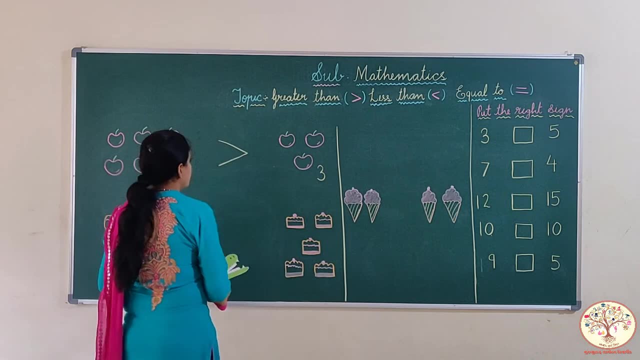 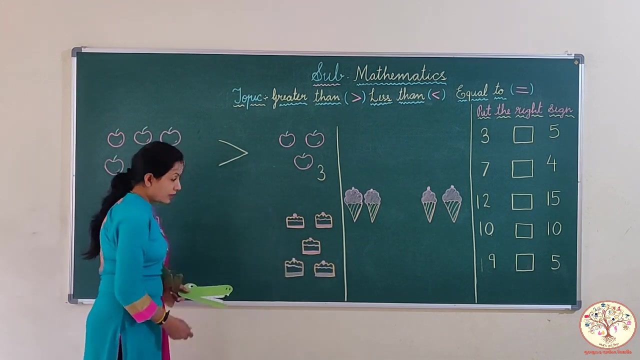 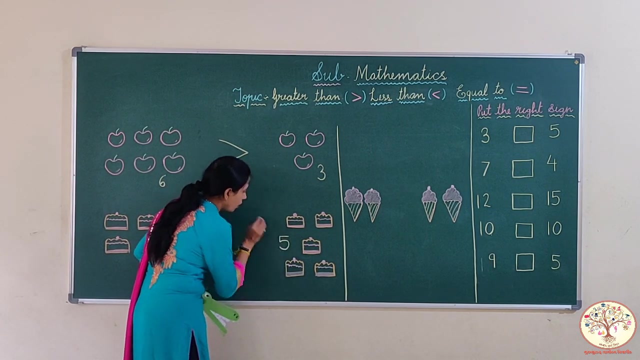 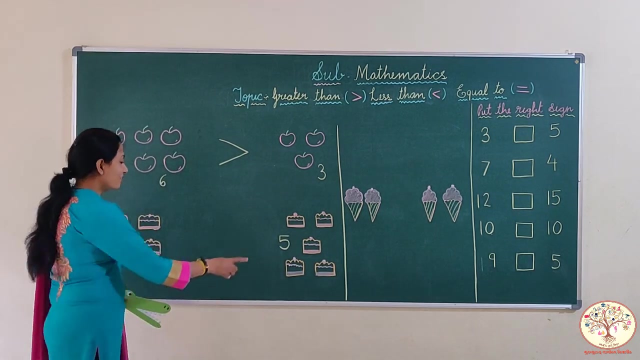 Four cakes. Here we have four cakes. Now count this side, One, two, three, four, five. This side we have five cakes. So can you tell me which is bigger number, four or five? Five 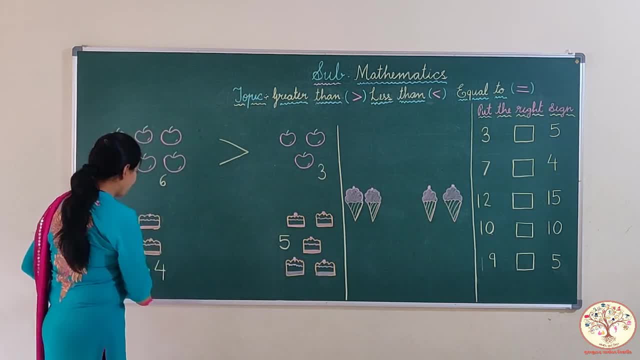 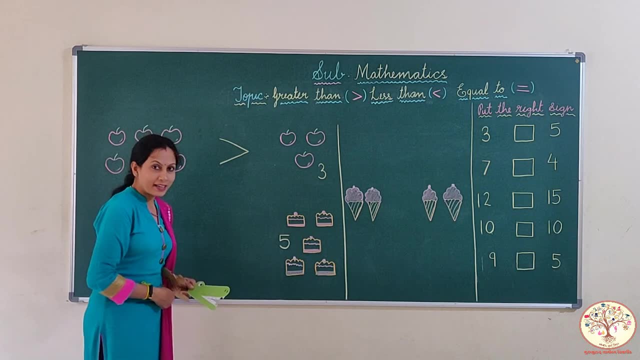 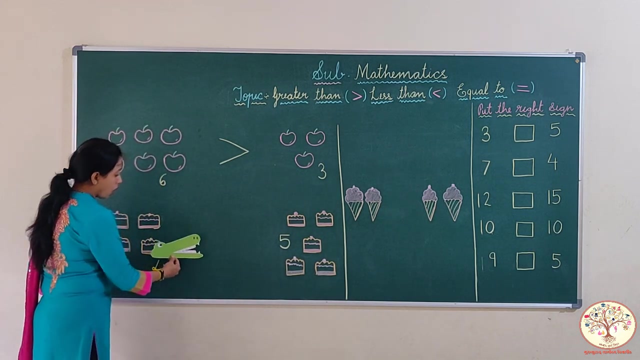 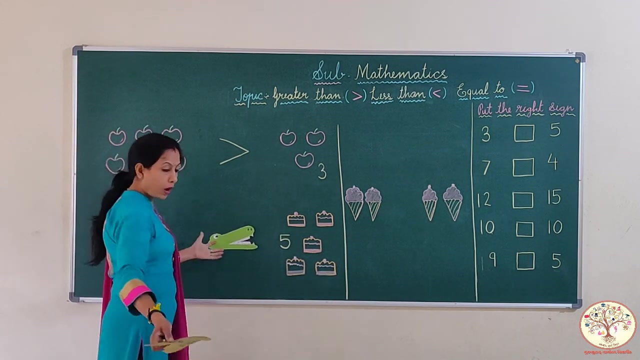 Yes, So Cuckoo will eat four cakes or five cakes. Five cakes Because Cuckoo is very hungry and he always eat more things, The bigger number. So now Cuckoo is going towards five cakes. Now you see where has Cuckoo's mouth opened. 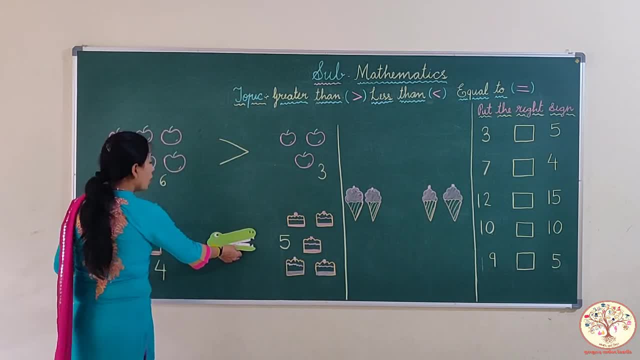 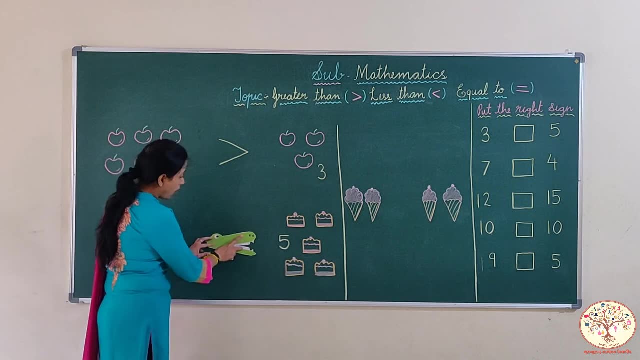 Towards five cakes, Because there are four cakes on this side. Four is less than five. Four is less than five. So now Cuckoo's mouth opens towards five cakes. So we put the sign of Cuckoo's mouth like this: 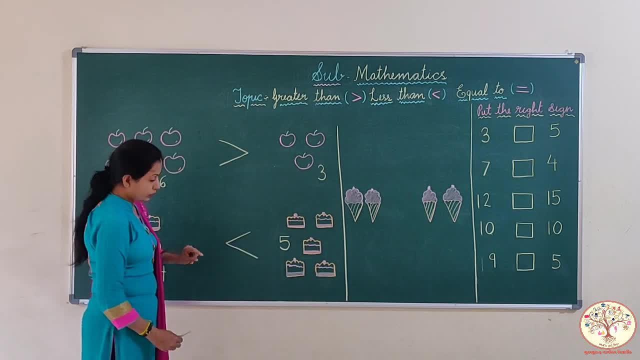 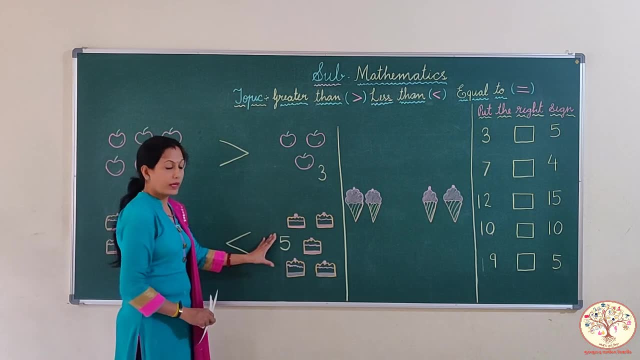 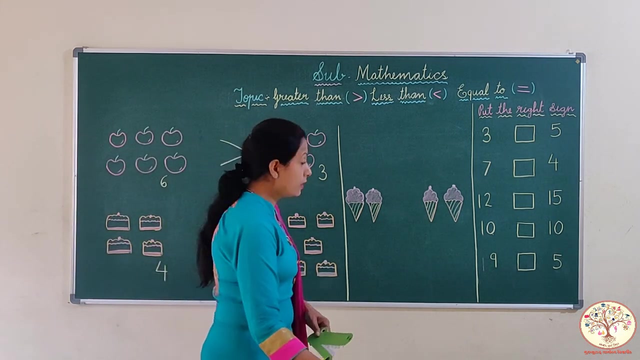 Okay, Now how is this sign? It is like Cuckoo's mouth: It is open towards more cakes. Okay, Towards more cakes. So Cuckoo ate more cakes. Now he finds some ice creams, Let's count them. 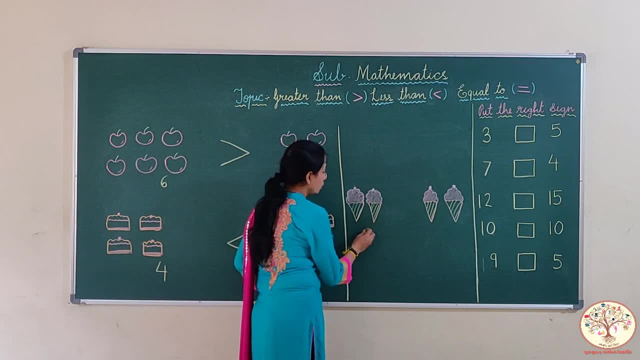 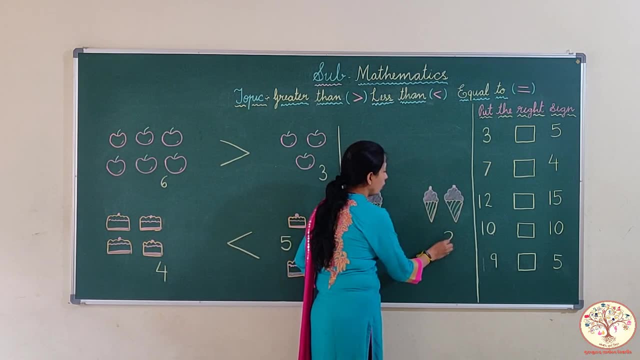 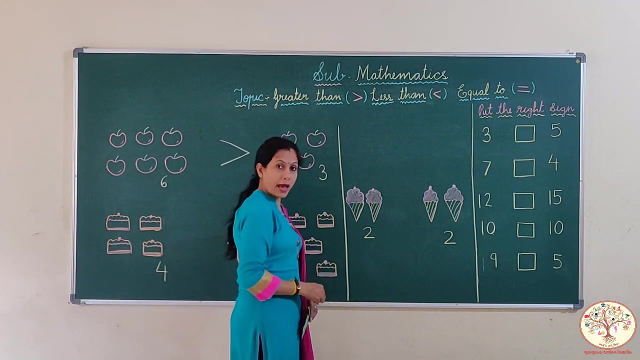 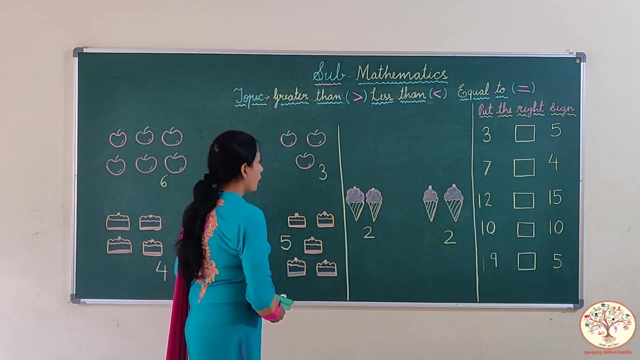 Here we have one two, Two ice creams And in this side one two, Two ice creams. Both sides we have the same number of ice creams. Okay, When Cuckoo sees the same number of things, it becomes confused. 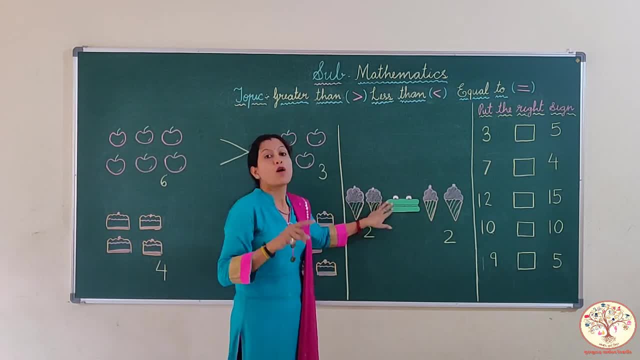 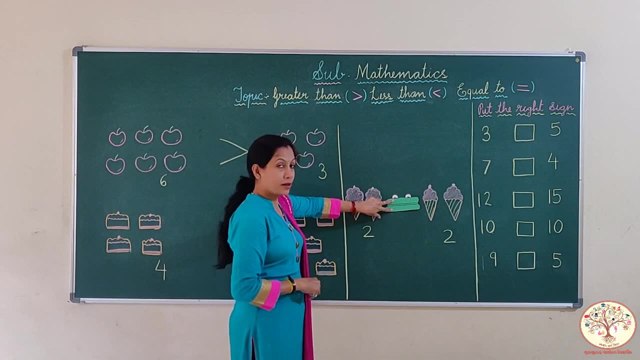 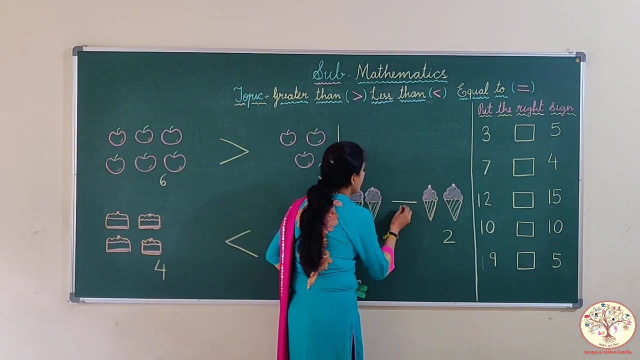 It becomes confused. It becomes confused and looks at us: Now, what should I eat? So Cuckoo becomes confused. Now how does his mouth look like? It looks like two lines. So how do we put this sign in the copy? 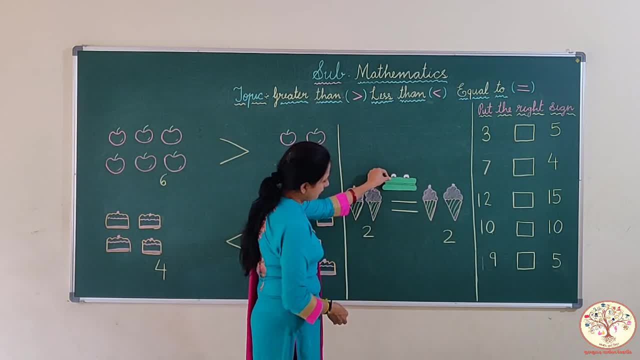 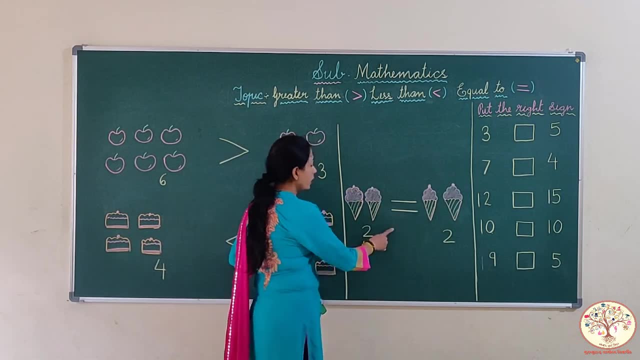 Two sleeping lines. You can see it like this: It is equal to Okay. What do we call this? Equal to Two, equal to two. Both sides have the same number. So which sign comes? Cuckoo's confused sign comes. 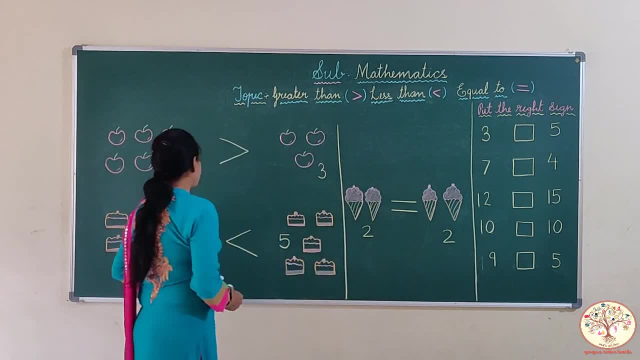 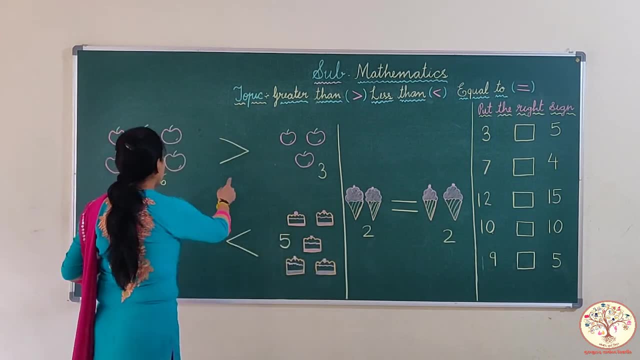 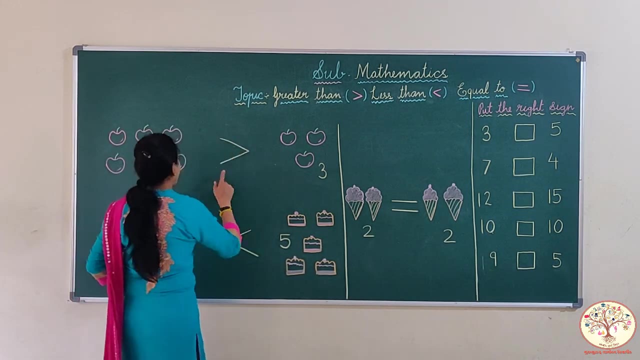 Two sleeping lines. So kids always see the things or the numbers on the left side and put the sign: When this side has more things, Cuckoo's mouth opens this side and we call it greater than. What do we call this sign? 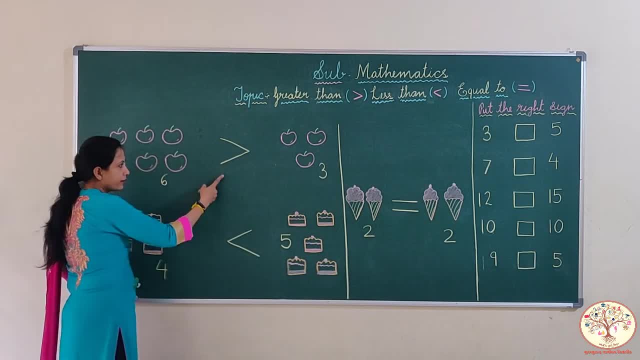 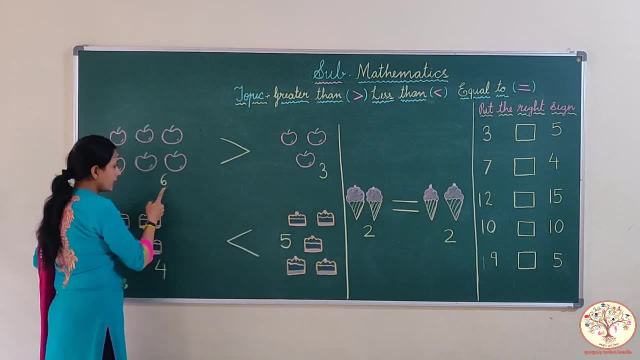 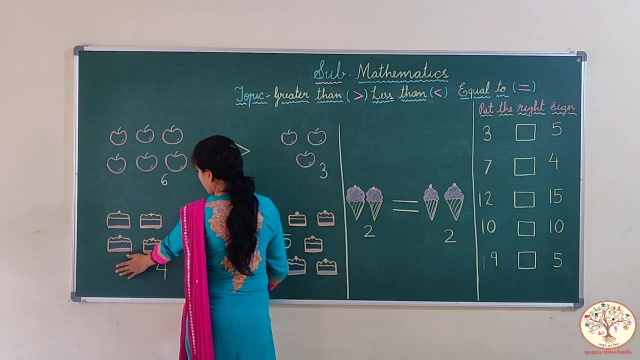 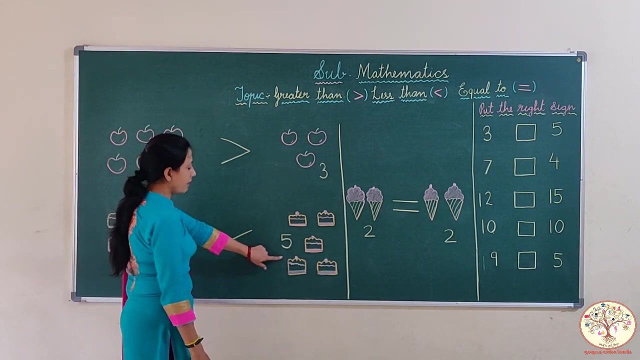 Greater than We can say. six is greater than three, Six is greater than three, Six is greater than three. Now again, look on the left side. Four, Okay, And in this side we have five. So we call this sign less than. 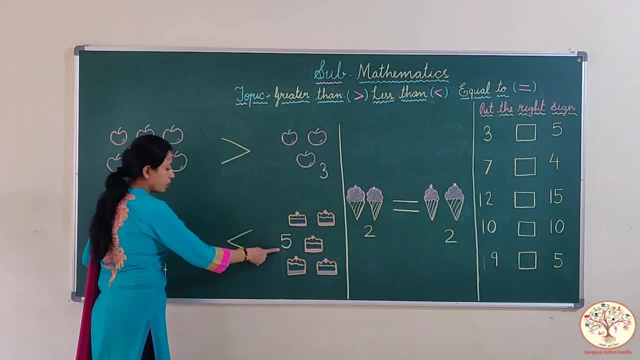 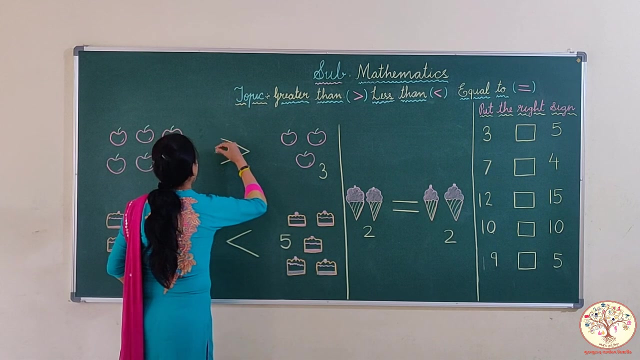 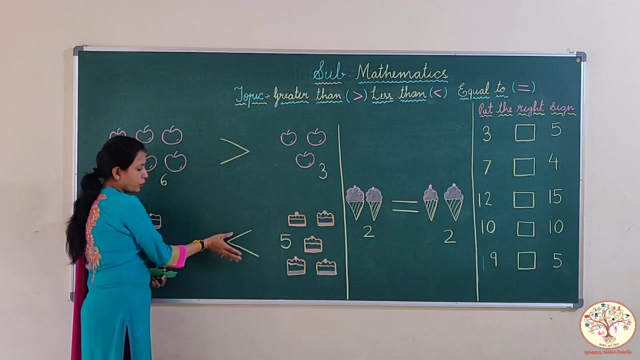 Four is less than five. Four is less than Four is less than. Four is less than five. Four is less than five. When Cuckoo's open its mouth towards left, we call it greater than When it opens its mouth towards right. 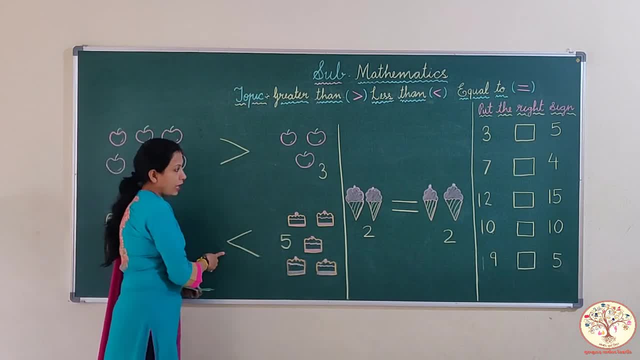 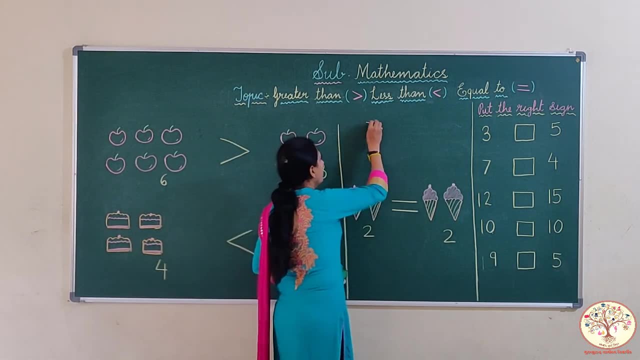 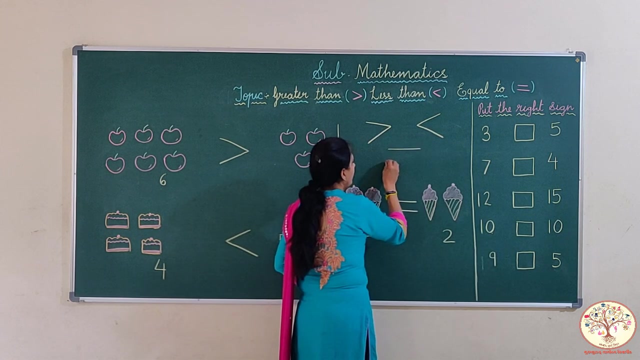 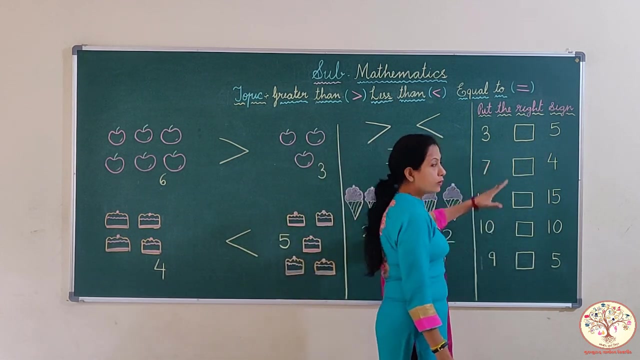 we call it less than, And this is the sign of equal to. We learnt three signs: Okay: Greater than, Less than And equal to. So now we will compare these numbers and put the right sign in the box. Okay, 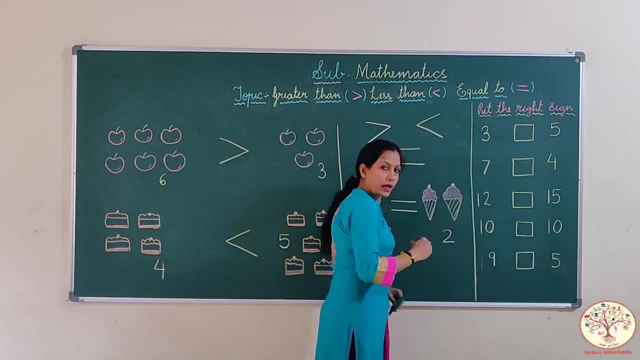 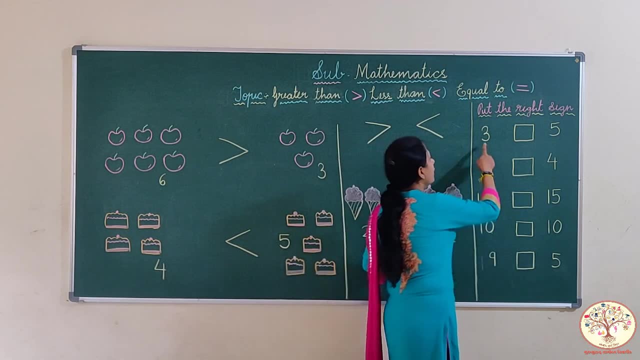 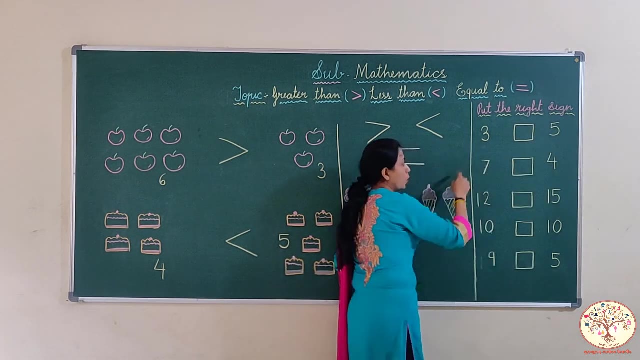 Now we will compare these numbers, Which one is bigger, Which one is smaller, And then we will put the right sign. Okay, So let's start This, sign number three, And on this side, number five. So which one is bigger? 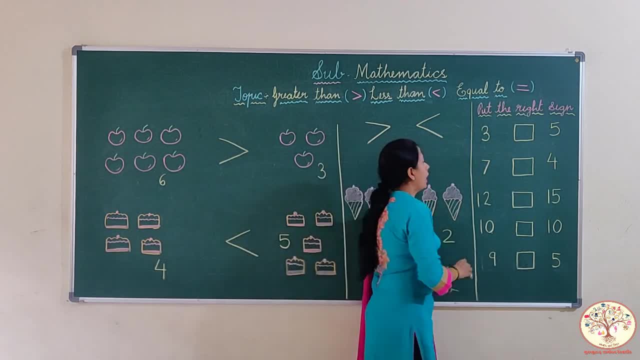 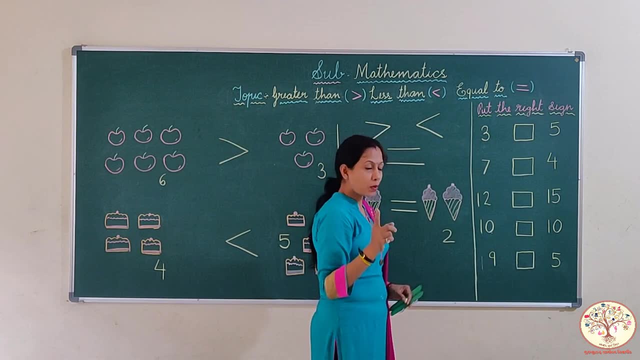 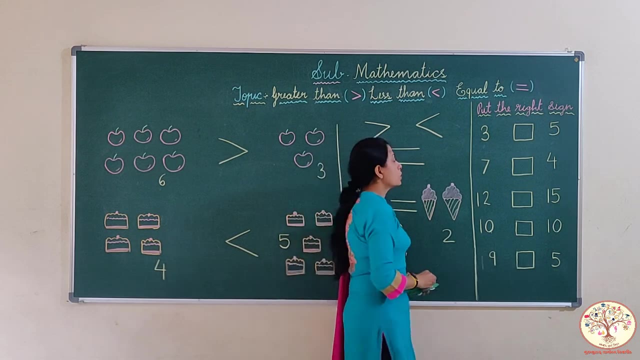 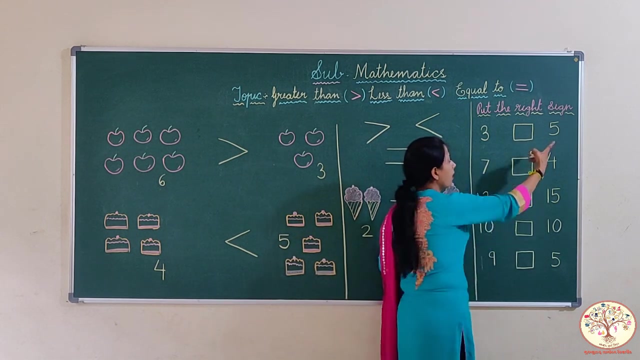 Can you tell me? I told you the number that comes first in counting That is smaller number, Okay. So one, two, three, Three comes first. Okay, So three is less than five. Okay. So where will crocodile's mouth be? 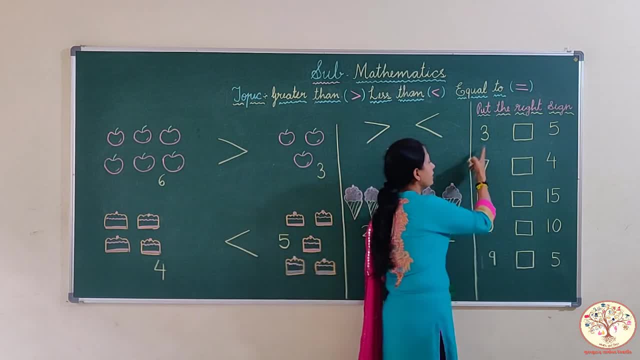 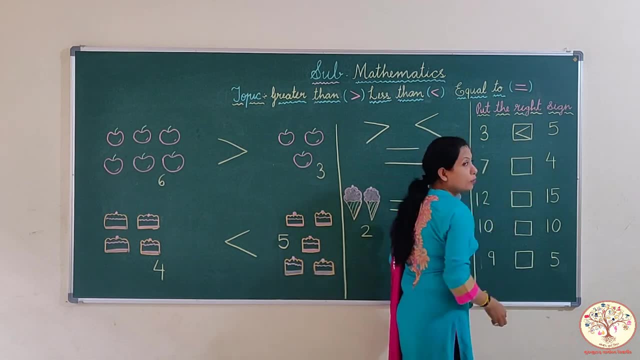 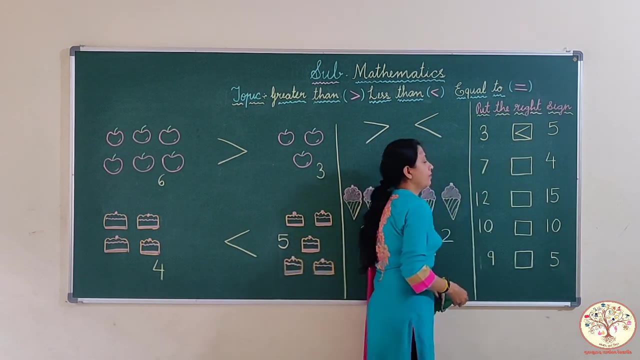 Towards five. Five is bigger number And three is smaller. Three is smaller number, So crocodile's mouth will be open towards five. And what do we call this? Less than Three is less than five. Now look at here. 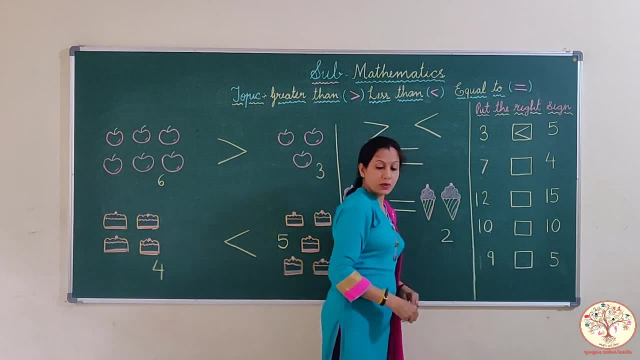 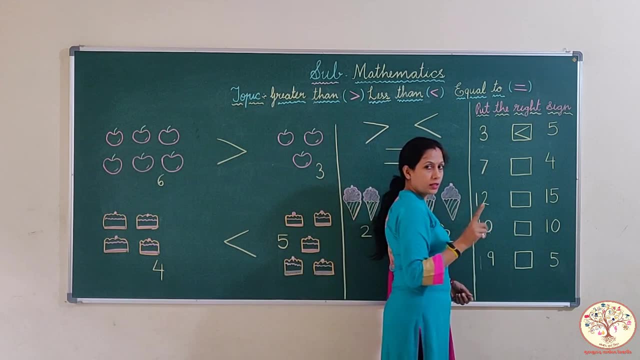 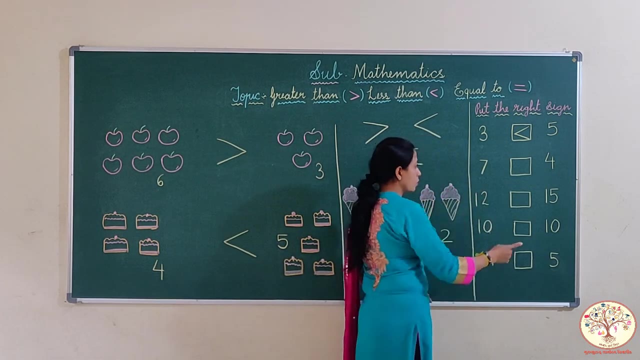 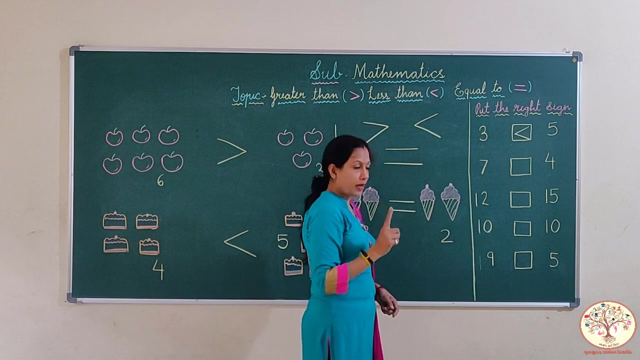 Seven and four. Which one is big and which one is small? Let's count. The number comes first in counting We call it smaller number One, two, three, four. So four is smaller number than seven. Seven is big and four is small. 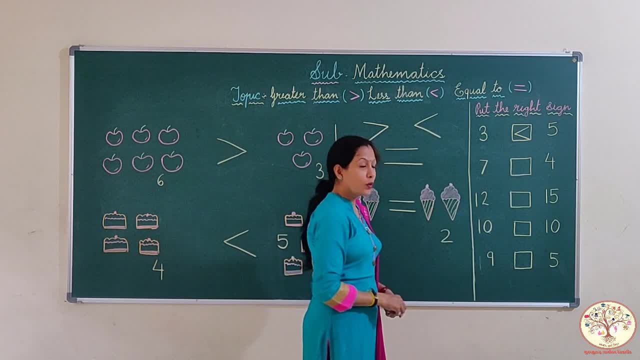 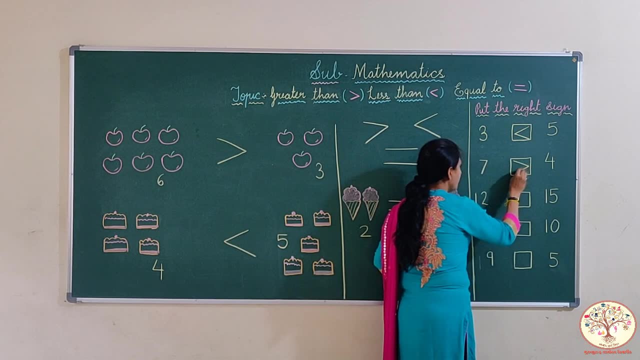 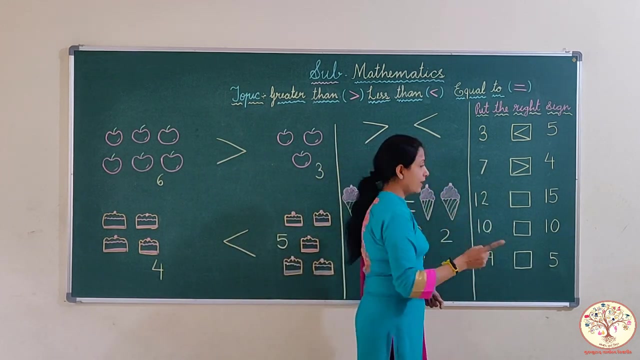 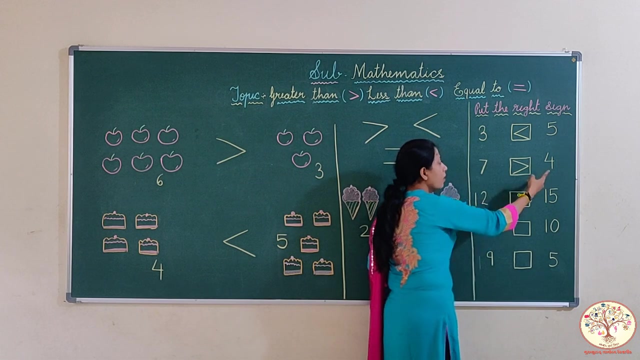 So which number will crocodile eat? Yes, Seven. So crocodile's mouth open towards seven. Okay, And what do we call this sign? Greater than Seven is greater than four. Seven is bigger than four. Okay, Now look here. 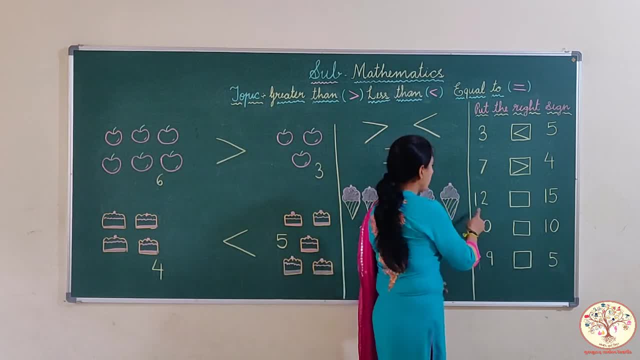 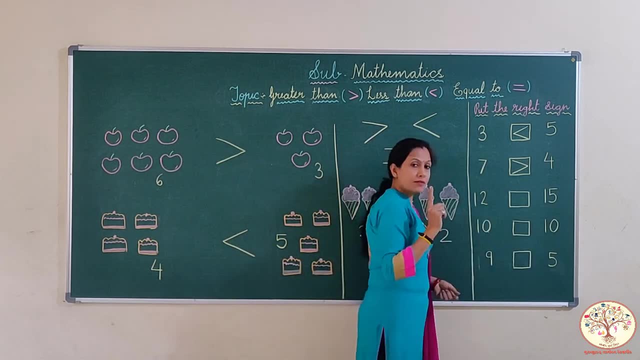 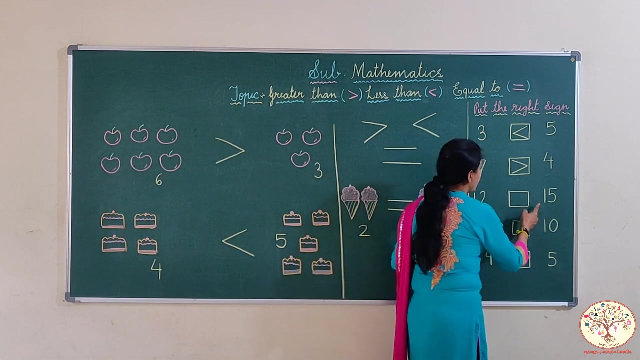 Here we have two digit numbers, One, two, twelve, One, five, fifteen In two digit number. first we look at tens place. Okay, Let's look at tens place. Tens place has the same number, One, one. 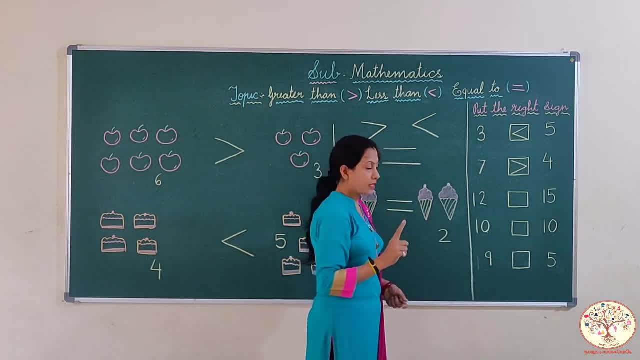 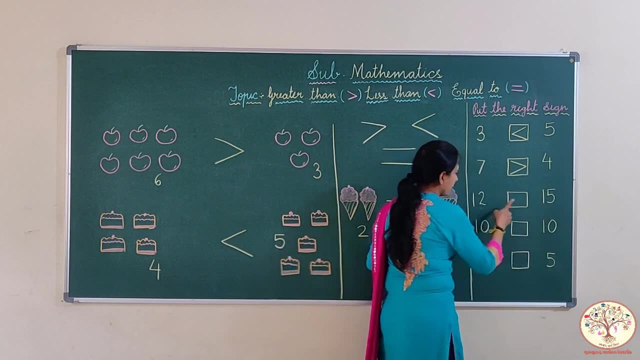 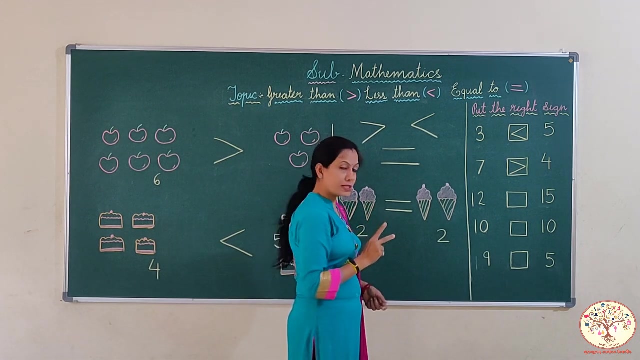 Now we look at ones place. Now let's look at ones place. Here we have two and five, Two and five. Comparing two and five, Which one is bigger and which one is smaller. One, two, Two comes first. 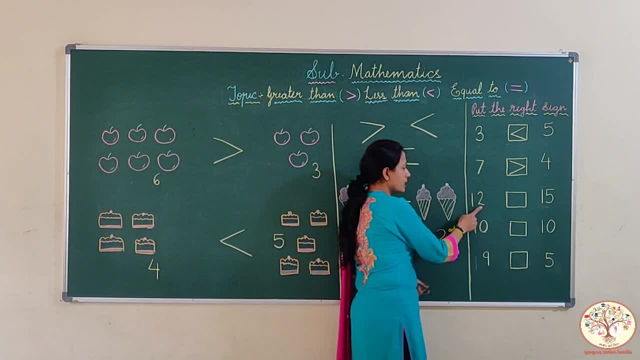 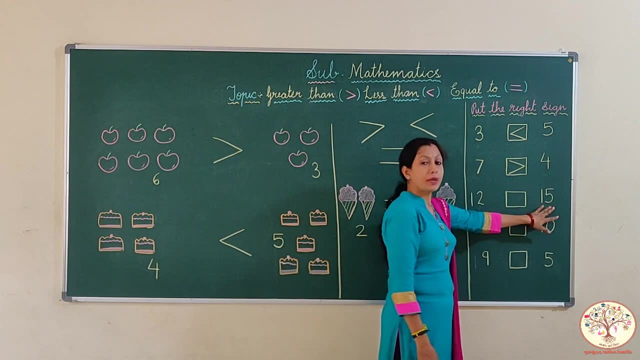 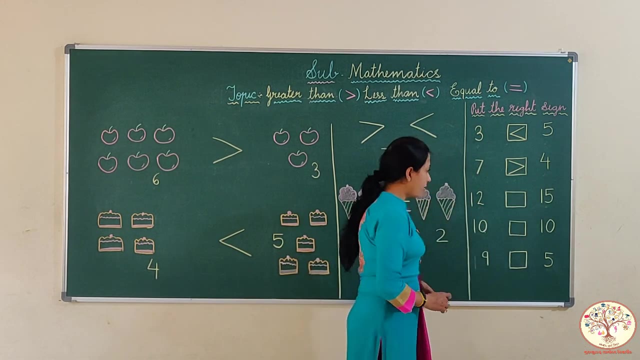 Two is smaller, So one. two, twelve is smaller than one. five, fifteen, Twelve is smaller than fifteen, So which one is bigger? Fifteen? This one is smaller and this one is bigger, So crocodile will eat bigger number. 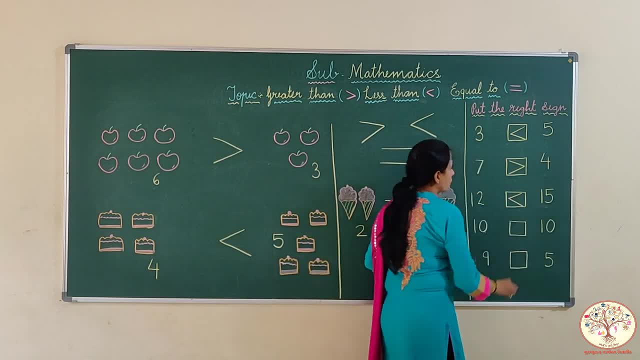 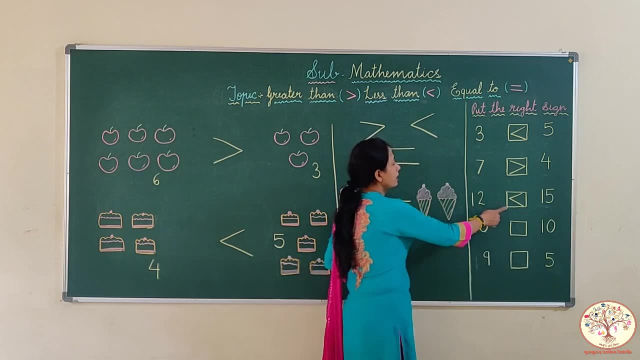 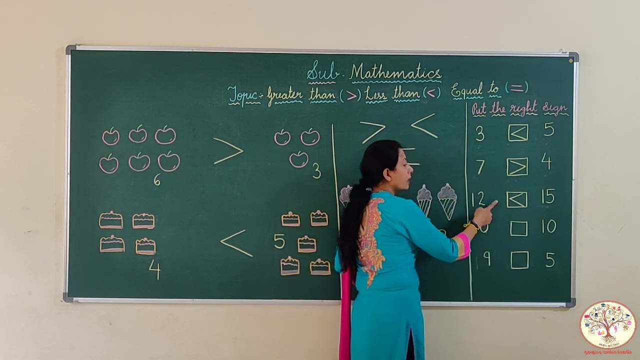 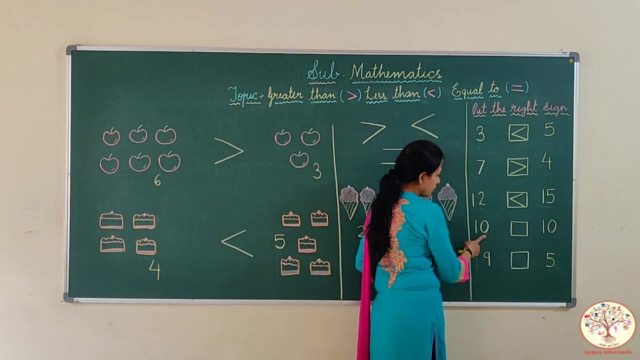 Its mouth open towards fifteen. Where is crocodile's mouth open Towards fifteen? Okay, We call it less than sign. Twelve is less than fifteen. Twelve is smaller than fifteen. Okay, Now look at these numbers. One zero ten. 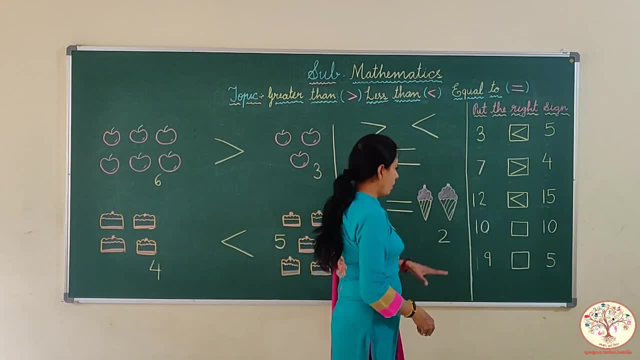 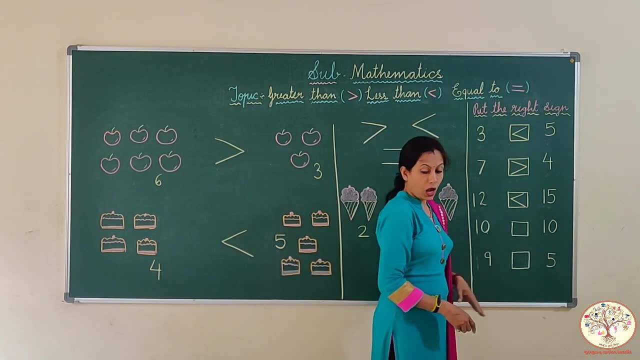 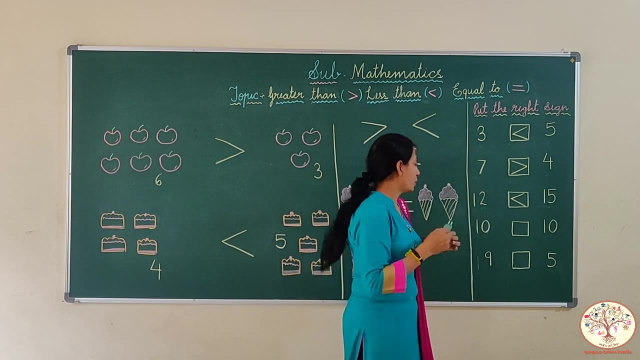 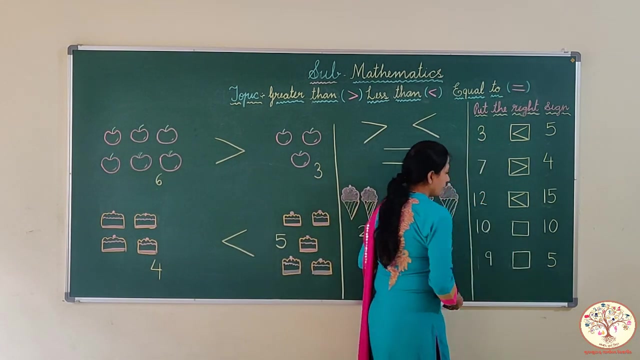 On this side one, zero, ten. Both side have same numbers. Ten, ten. Now crocodile get confused. Hmm, Like this right. So which sign we will put here? Equal to? When both side has same number, we put the sign of equal to. 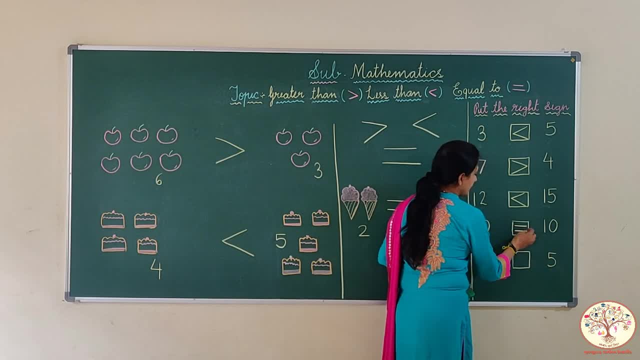 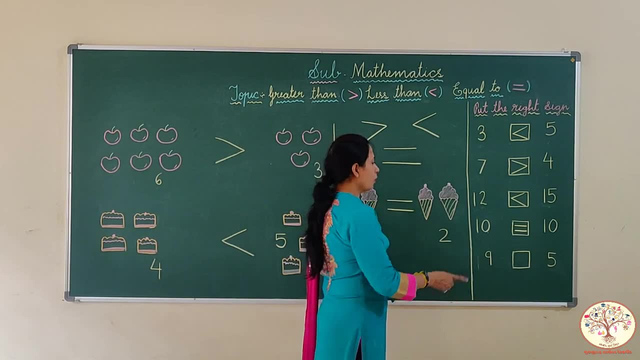 Two sleeping lines Equal to ten is equal to ten, Ten and ten are equal, No big and no small. Now look at this number: nine And on this side five. So can you tell me which one is smaller and which one is bigger? 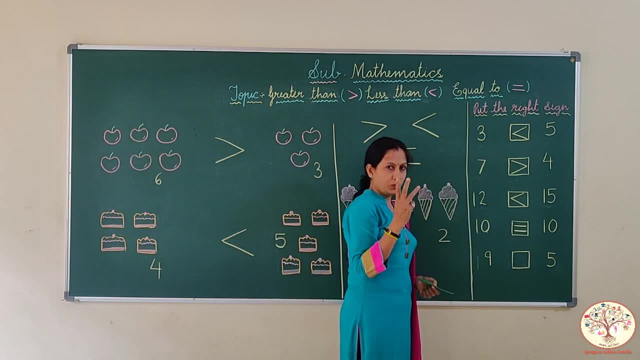 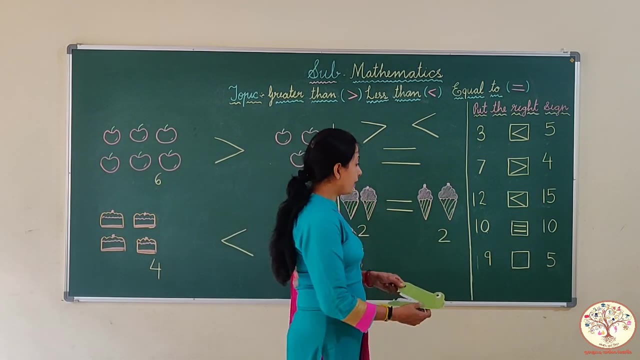 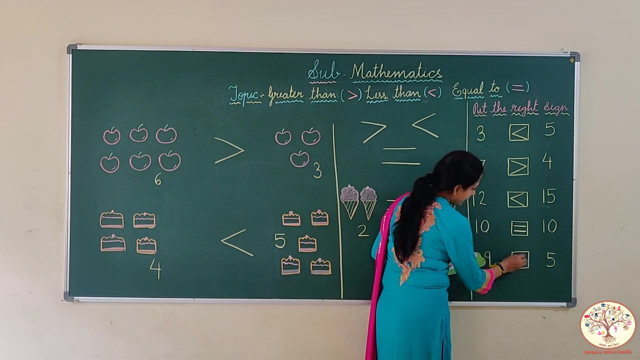 Okay, Let's count One, two, three, four, five. Five comes first, Five is smaller And nine is bigger, So crocodile will eat. Who will crocodile eat? Nine? Okay, So we will put the sign like this: 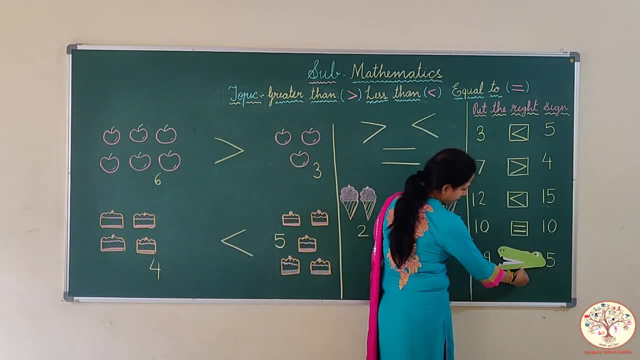 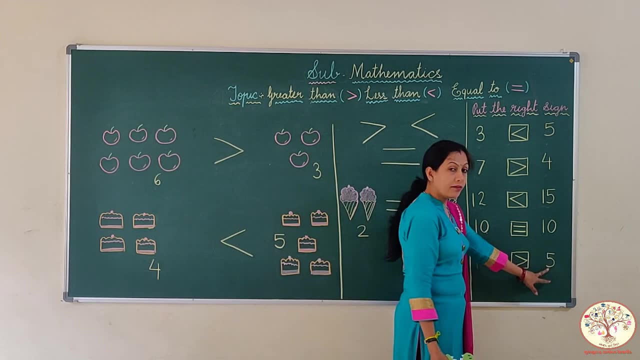 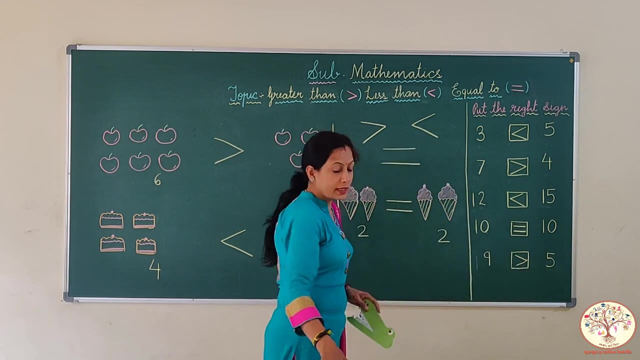 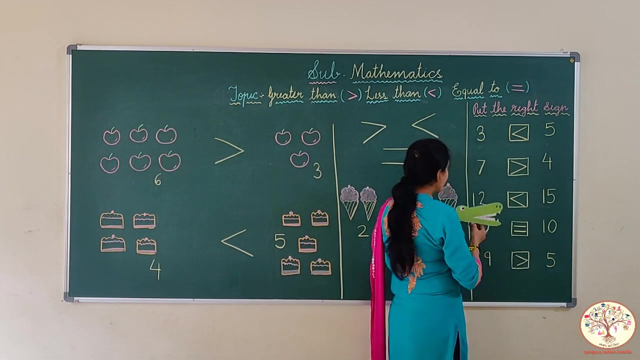 Which side is crocodile's mouth open? See Towards nine. So we say nine is greater than five. Nine is bigger than what Five? So look here, kids, Match the sign Three and five. Five is bigger. So crocodile will eat number five. 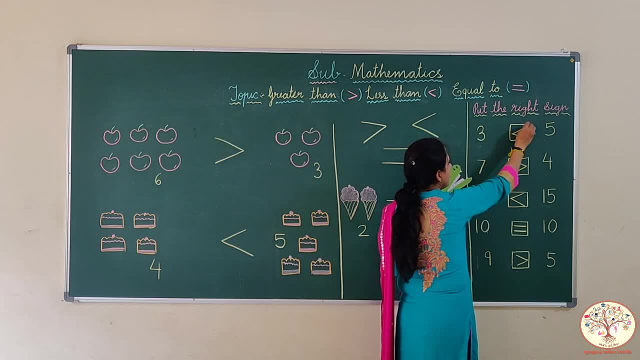 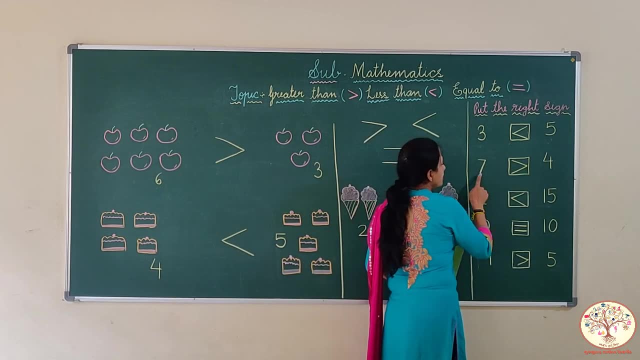 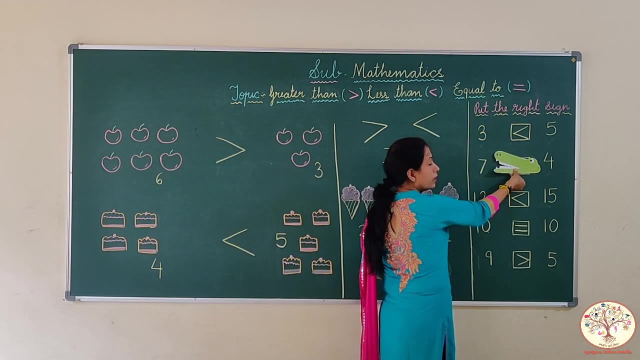 We put the sign like this: Open side towards bigger number, Okay, And in this we have seven this side and four on this side, So crocodile will eat seven, The bigger number. Crocodile is always very hungry, He eats bigger number. 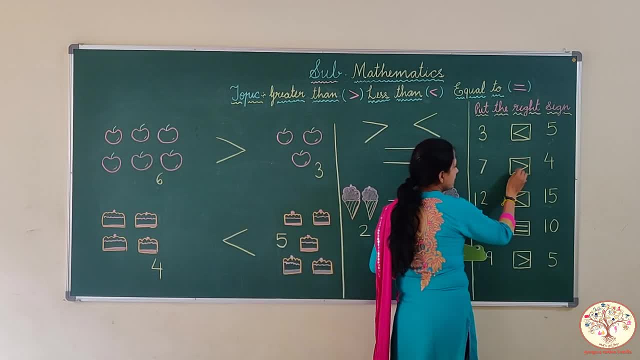 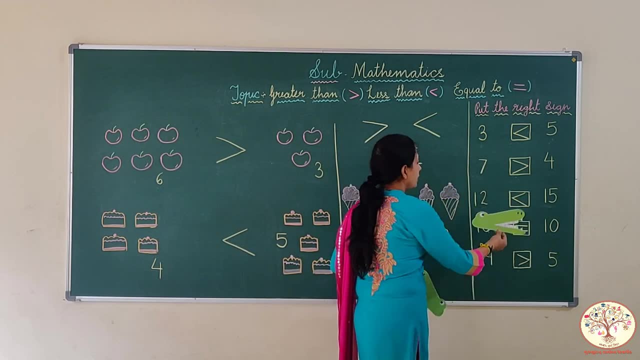 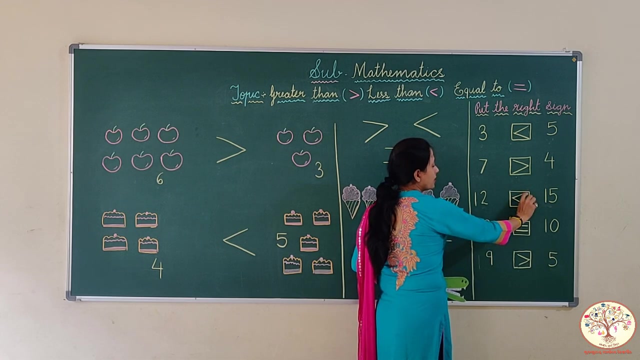 Okay. So we put the sign like this: Open side towards seven, Twelve and fifteen Crocodile will eat fifteen. We put the sign like this: Open side towards fifteen And in ten, crocodile get confused. We put the sign of equal to.